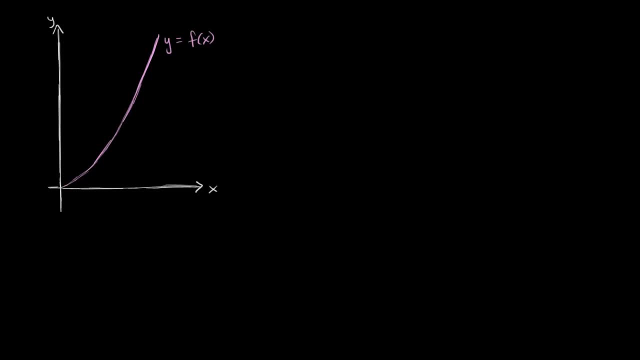 We've used definite integrals to find areas. What I want to do now is to see if we can use a definite integral to find an arc length. What do I mean by that? Well, if I start at this point, on the graph of a function. 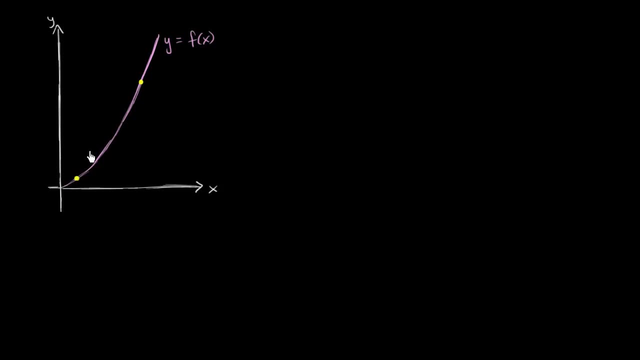 and if I were to go to this point right over here, not in a straight line- we know already how to find the distance in a straight line- but instead we want to find the distance along the curve. If we were to lay a string along the curve? what would be this distance right over here? That's what I'm talking about by arc length. We could think about it as: okay, well, that's going to be from x equals a to x equals b along this curve. How could we do it? 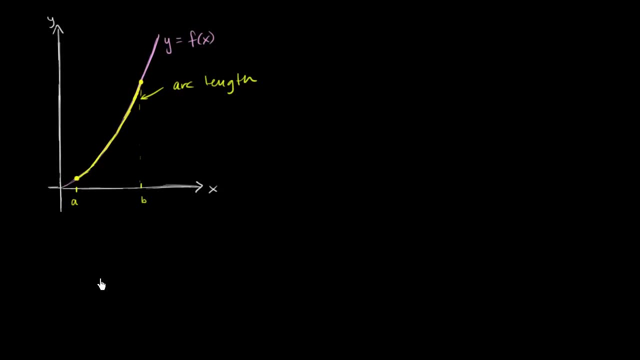 Well, the one thing that integration integral calculus is teaching us is that when we see something that's changing like this, what we can do is we can break it up into infinitely small parts, infinitely small parts that we can approximate it with things like lines and rectangles. 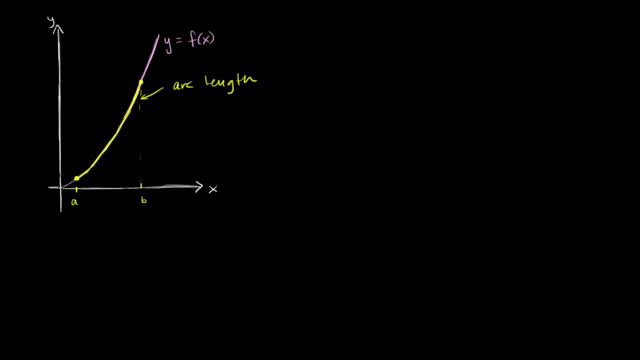 and then we could take the infinite sum of those infinitely small parts. Let me break up my arc length into infinitely small sections of arc length. Let me call each of those infinitely small sections of my arc length a length of differential, an arc length of differential. 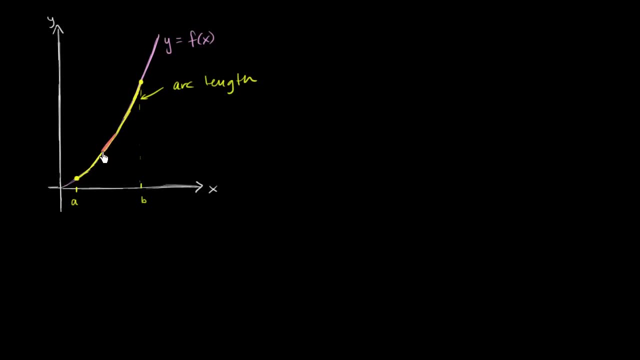 I'll call it ds. I'm going to draw it much bigger than when. at least I conceptualize what a differential is, just so that we can see it. What do I mean by breaking it up into these ds's? Well, if that's a ds. 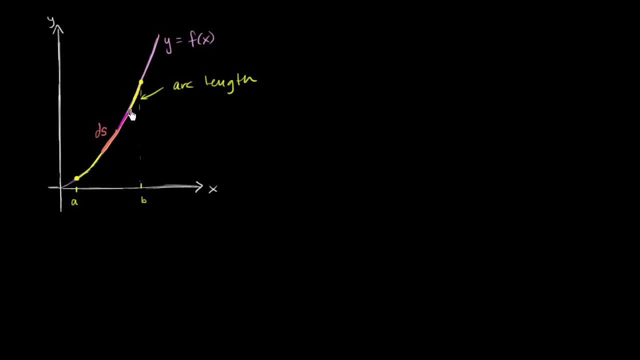 and then let me do these others in another color. that's another change- infinitely small change in my arc length. another infinitely small change in my arc length. If I summed all of these ds's together, I'm going to get the arc length. 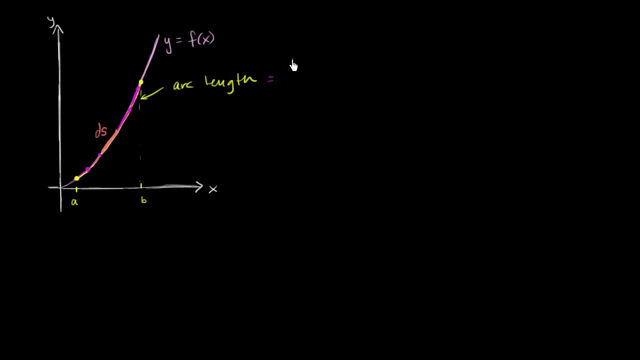 The arc length, if I take, is going to be the integral of all of these ds's, All of these ds's sum together over this interval. We can denote it like this- This doesn't help me right now. This is, in terms of this arc length, differential. 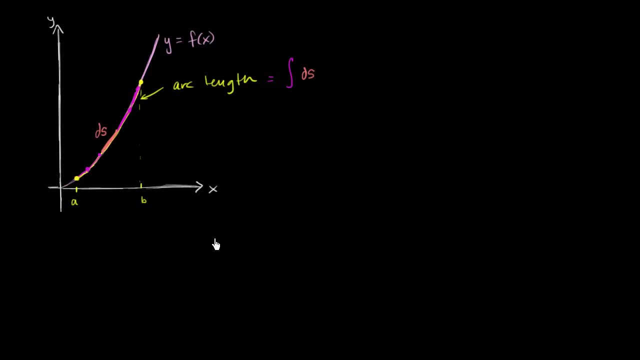 We know how to do things in terms of dx's and dy's. Let's see if we can re-express this in terms of dx's and dy's If we go on a really, really small scale. once again, we can approximate. 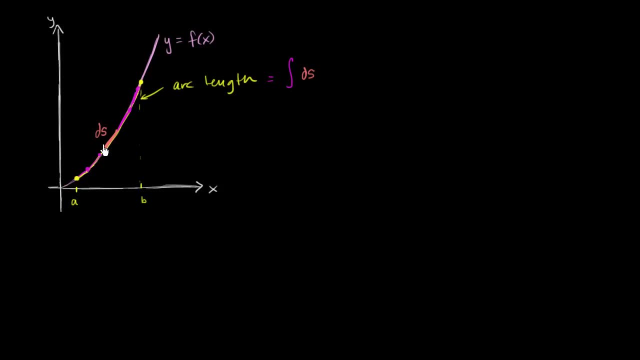 This is going to be a line, just the way that we approximated area with rectangles at first. but if you have an infinite number of infinitely small rectangles, you're actually approximating a non-rectangular region, the area of a non-rectangular region. 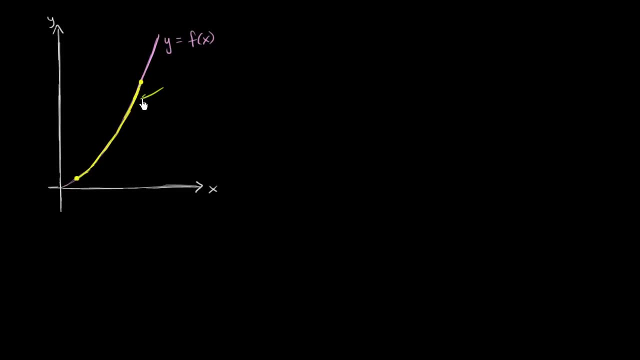 what would be this distance right over here? That's what I'm talking about by arc length. We could think about it as: okay, well, that's going to be from x equals a to x equals b along this curve. How could we do it? 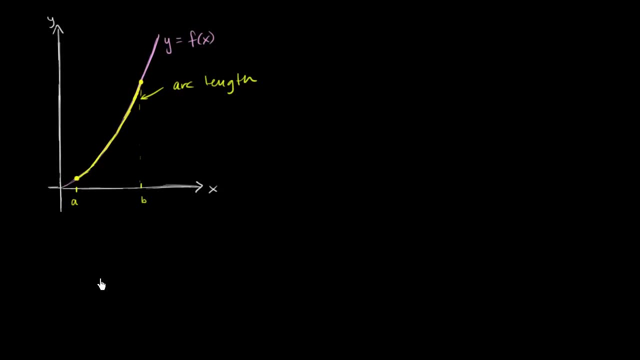 Well, the one thing that integration integral calculus is teaching us is that when we see something that's changing like this, what we can do is we can break it up into infinitely small parts, infinitely small parts that we can approximate it with things like lines and rectangles. 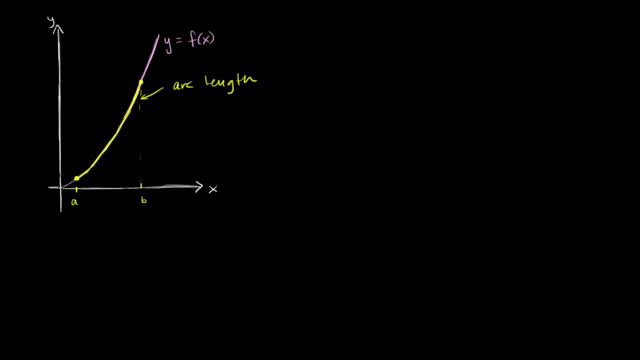 and then we could take the infinite sum of those infinitely small parts. Let me break up my arc length into infinitely small sections of arc length. Let me call each of those infinitely small sections of my arc length a length of differential, an arc length of differential. 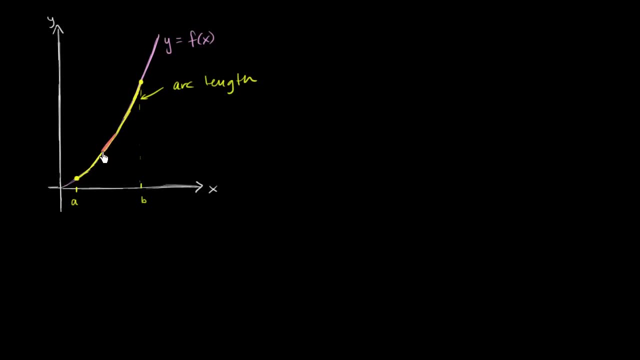 I'll call it ds. I'm going to draw it much bigger than when. at least I conceptualize what a differential is, just so that we can see it. What do I mean by breaking it up into these ds's? Well, if that's a ds. 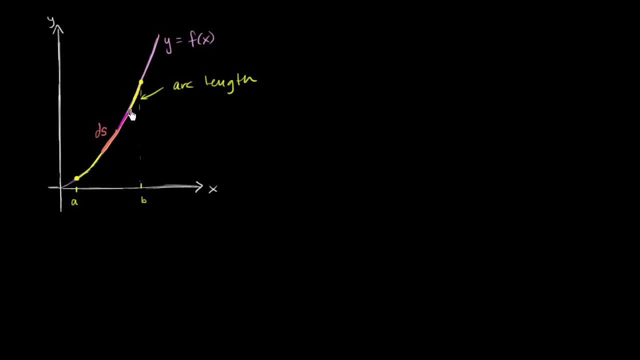 and then let me do these others in another color. that's another change- infinitely small change in my arc length. another infinitely small change in my arc length. If I summed all of these ds's together, I'm going to get the arc length. 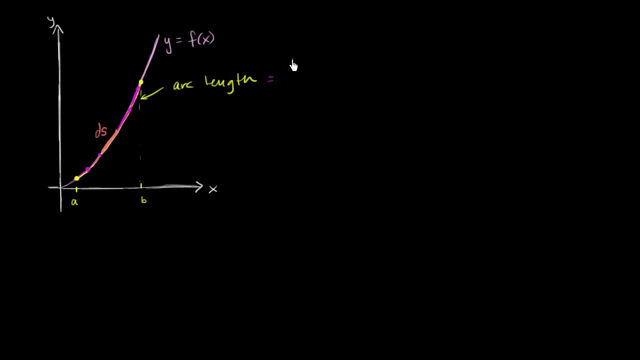 The arc length, if I take, is going to be the integral of all of these ds's, All of these ds's sum together over this interval. We can denote it like this- This doesn't help me right now. This is, in terms of this arc length, differential. 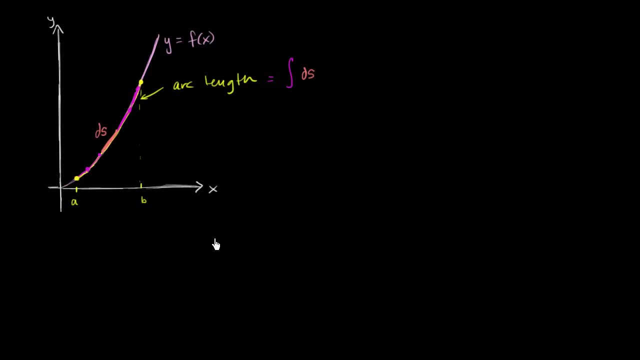 We know how to do things in terms of dx's and dy's. Let's see if we can re-express this in terms of dx's and dy's If we go on a really, really small scale. once again, we can approximate. 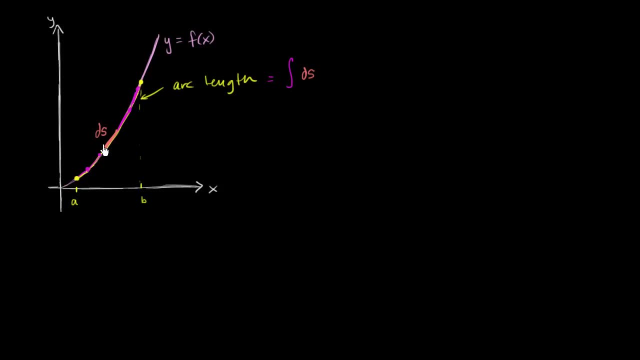 This is going to be a line, just the way that we approximated area with rectangles at first. but if you have an infinite number of infinitely small rectangles, you're actually approximating a non-rectangular region, the area of a non-rectangular region. 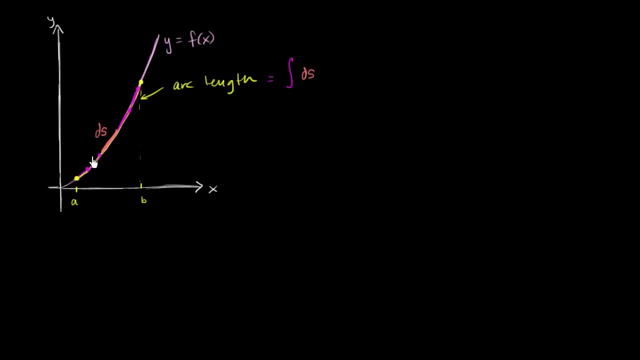 Similarly, we're approximating with lines here, but they're infinitely small and there's an infinite number of them. you are actually finding the length of the curve Just focusing on this as a line for now, This distance right over here. I'm just going to try to express it. 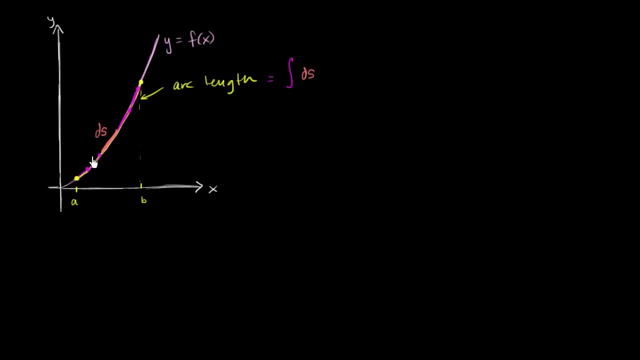 Similarly, we're approximating with lines here, but they're infinitely small and there's an infinite number of them. you are actually finding the length of the curve Just focusing on this as a line for now, This distance right over here. I'm just going to try to express it. 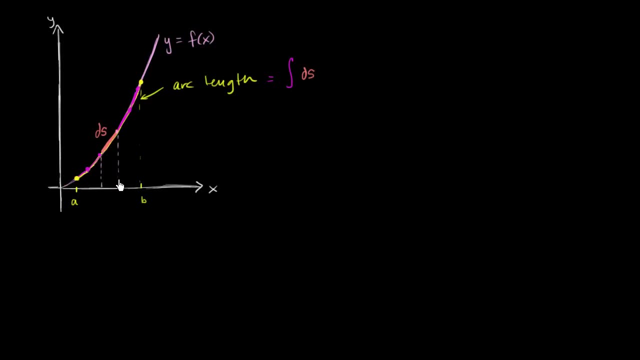 in terms of dx's and dy's. This distance right over here, that's dx. You can view this as an infinitely small change in x. This distance right over here, this is a dy. Once again, I'm being loosey-goosey. 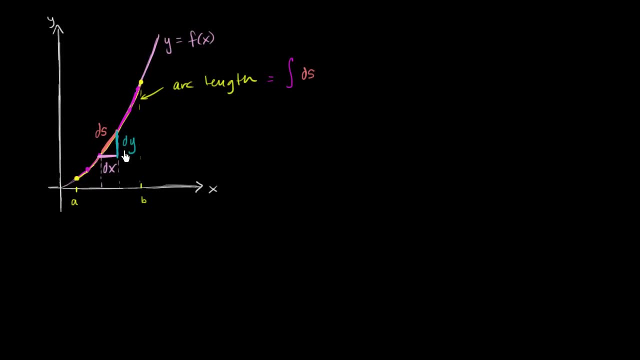 with differentials, really to give you conceptual understanding, not a rigorous proof, but it'll give you a sense of where the formula for arc length is actually coming from. Based on this, you can see that ds could be expressed based on the Pythagorean theorem. 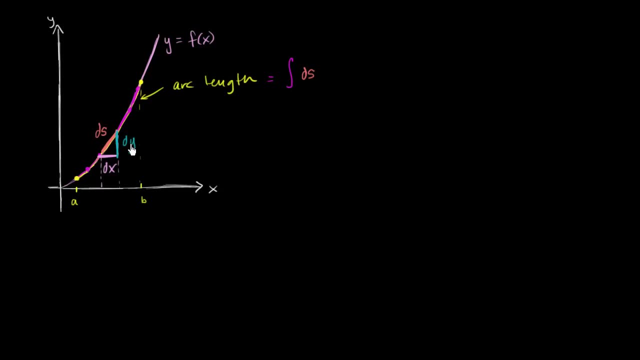 as equal to dx squared plus dy squared. Or you could rewrite it as the square root of dx squared plus dy squared. We can rewrite this. We could say: this is the same thing as the integral of. instead of writing ds, I'm going to write it as: 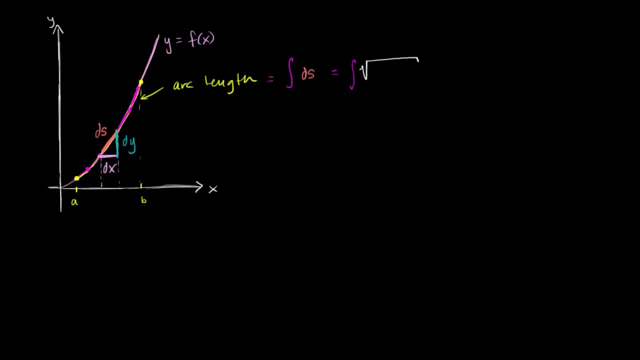 the square root of dx squared plus dy squared Once again. this is straight out of the Pythagorean theorem. Now this is starting to get interesting. I've written in terms of dx's and dy's, but they're getting squared, they're under a radical sign. 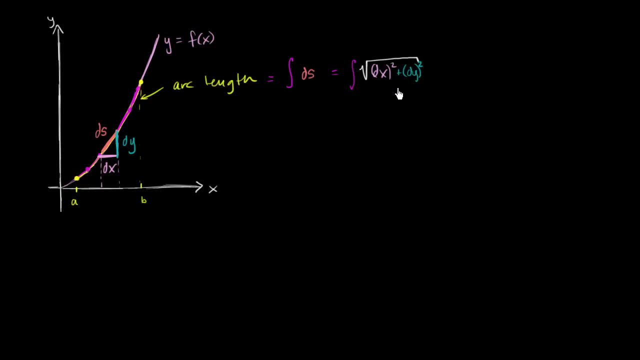 What can I do to simplify this, Or at least write it in a way that I know how to integrate? Well, I could factor out a dx squared, So let me just rewrite it. This is going to be the same thing as the integral of the square root. 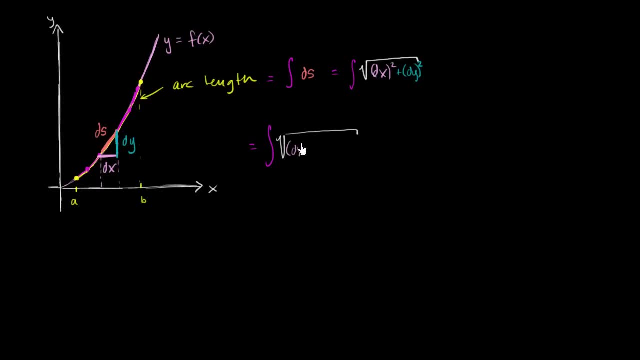 I'm going to factor out a dx squared, dx squared times 1 plus dy over dx squared. Notice this. and this is the exact same quantity If I distribute this dx squared. I'm going to get this right up here, And now I can take the dx squared. 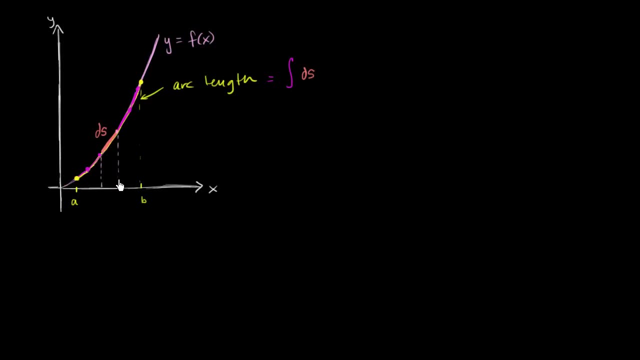 in terms of dx's and dy's. This distance right over here, that's dx. You can view this as an infinitely small change in x. This distance right over here, this is a dy. Once again, I'm being loosey-goosey. 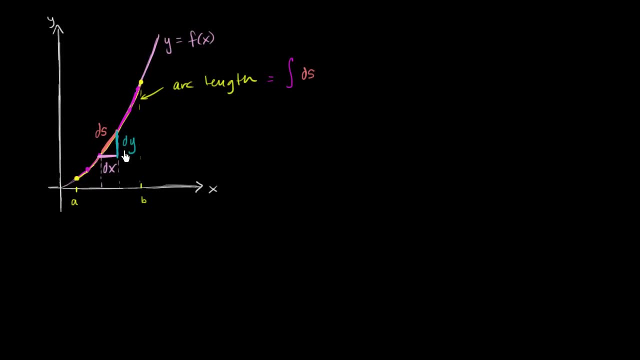 with differentials, really to give you conceptual understanding, not a rigorous proof, but it'll give you a sense of where the formula for arc length is actually coming from. Based on this, you can see that ds could be expressed based on the Pythagorean theorem. 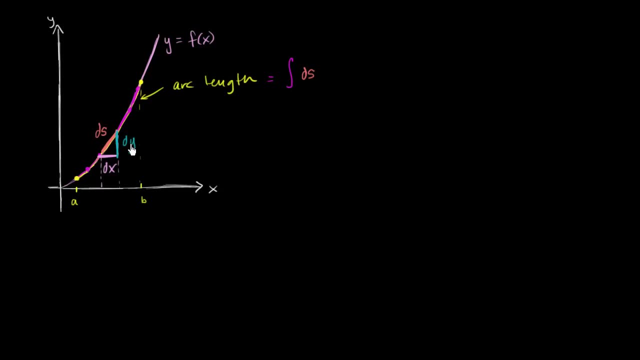 as equal to dx squared plus dy squared. Or you could rewrite it as the square root of dx squared plus dy squared. We can rewrite this. We could say: this is the same thing as the integral of. instead of writing ds, I'm going to write it as: 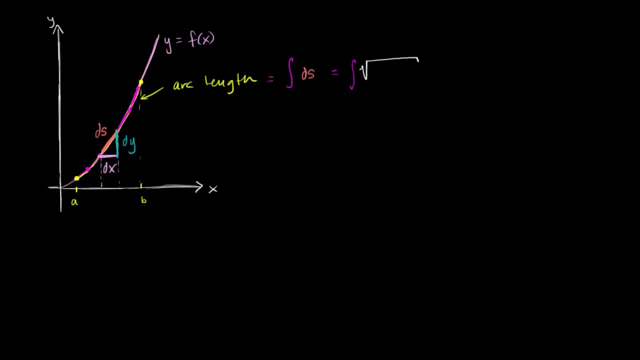 the square root of dx squared plus dy squared Once again. this is straight out of the Pythagorean theorem. Now this is starting to get interesting. I've written in terms of dx's and dy's, but they're getting squared, they're under a radical sign. 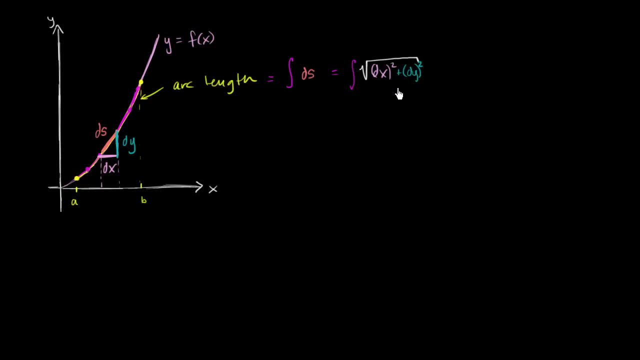 What can I do to simplify this, Or at least write it in a way that I know how to integrate? Well, I could factor out a dx squared, So let me just rewrite it. This is going to be the same thing as the integral of the square root. 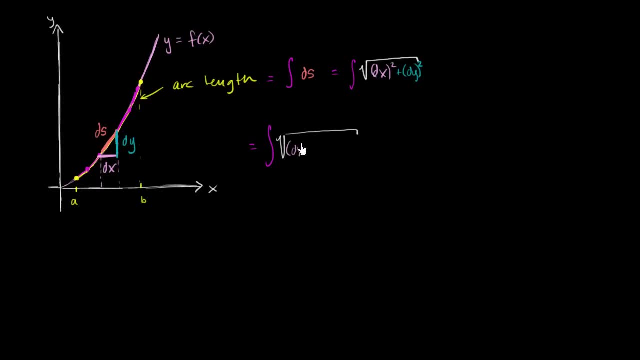 I'm going to factor out a dx squared, dx squared times 1 plus dy over dx squared. Notice this. and this is the exact same quantity If I distribute this dx squared. I'm going to get this right up here, And now I can take the dx squared. 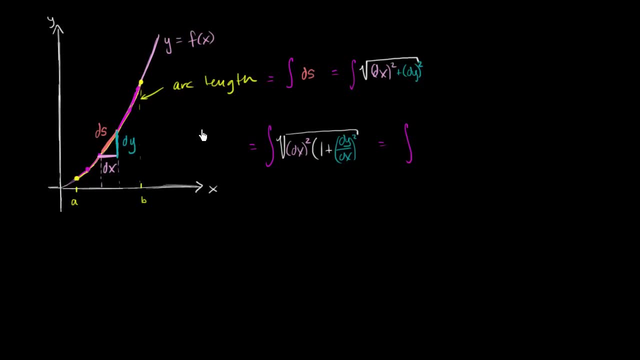 out of the radical, And so this is going to be, this is going to be the integral of. let me write that in that white color: the integral of 1 plus dy dx, squared, And this is interesting because we know what dy dx is.